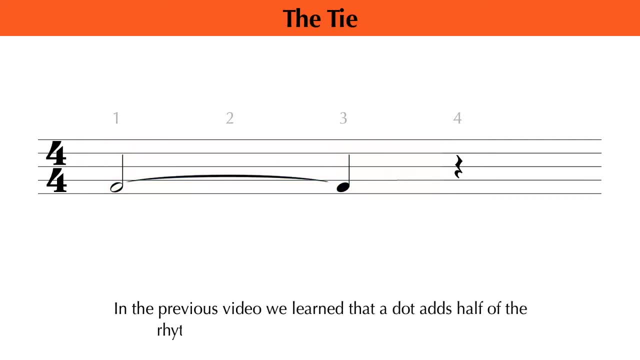 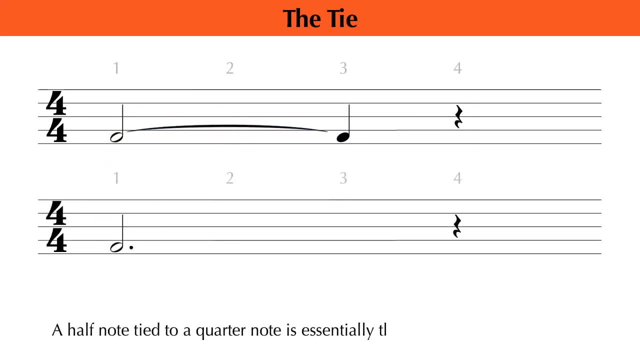 In the previous video we learned that a dot adds half of the rhythmic value of the note that it is attached to. A half note tied to a quarter note is essentially the same as is essentially the same as a dotted half note. Likewise, when a half note is tied to another half note. 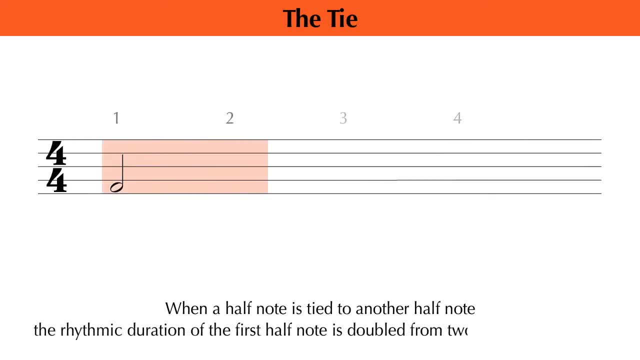 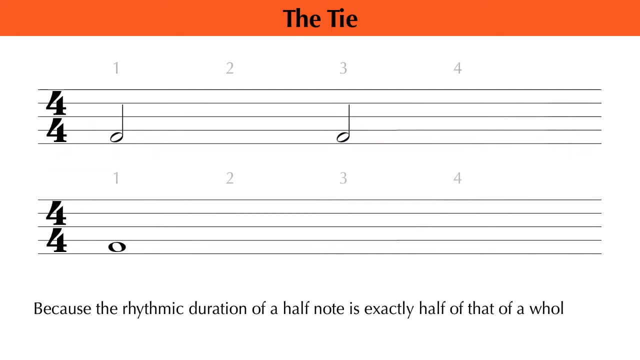 the rhythmic duration of the first half note is doubled from 2 beats to 4 beats Because the rhythmic duration of a half note is exactly half of that of a whole note. a half note tied to another half note is comparatively the same as a single whole note. 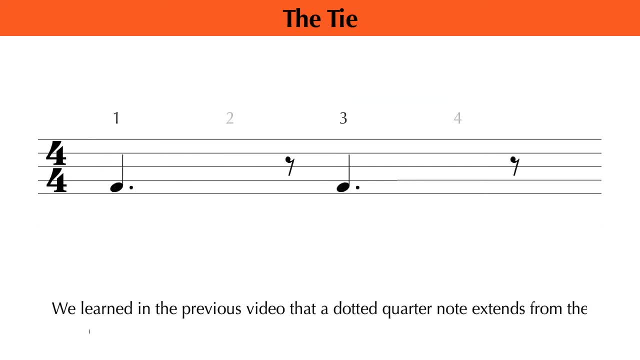 We learned in the previous video that a dotted quarter note extends from the down beat of a particular beat to the up beat of the following beat. This may also be achieved by tying each quarter note to an eighth note. We can see in this example that the quarter notes 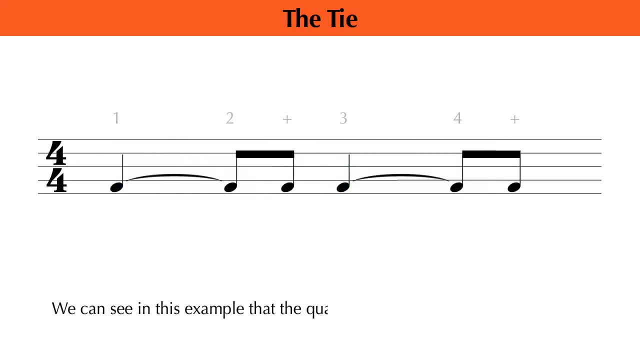 on beats 1 and 3 are tied to the first eighth note on the following beat. Being so, each quarter note will extend through the next down beat and the following note will be played on that up beat. Now it is important to remember that a tie. 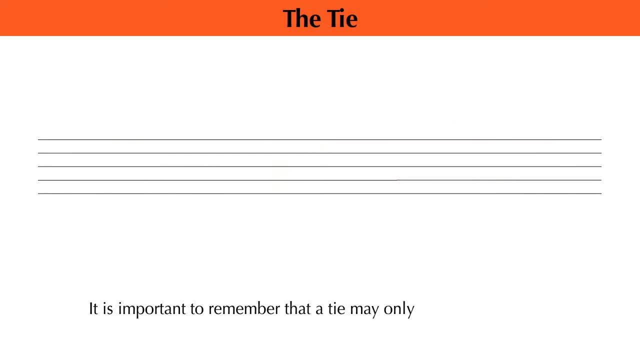 may only be used to connect two notes of equal pitch and letter name. For example, because these two notes are not on the same staff position, even though they are both the letter name F a tie may not be used to connect their rhythmic values. 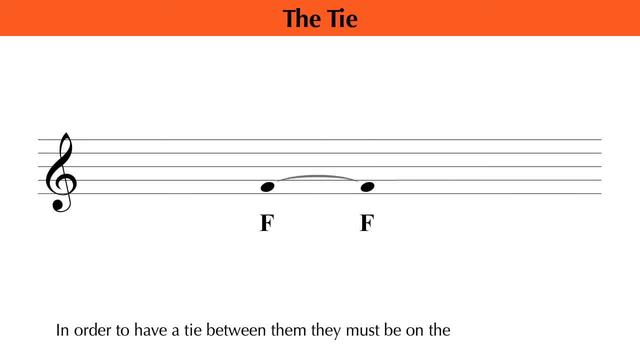 In order to have a tie between them, they must be on the same staff position. One of the many functional uses of a tie can be for when you want to extend the duration of a note past a measure line, For example, a half note placed on the fourth beat. 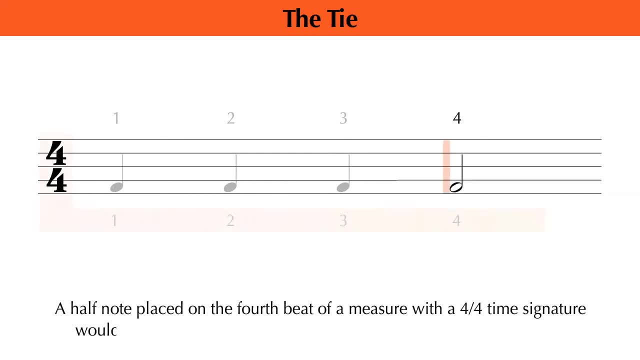 of a measure with a 4-4 time signature would extend the measure to five beats and would therefore not work. This can be fixed by replacing the half note with a quarter note and using a tie to connect it to a quarter note. on beat 1 of the following measure: